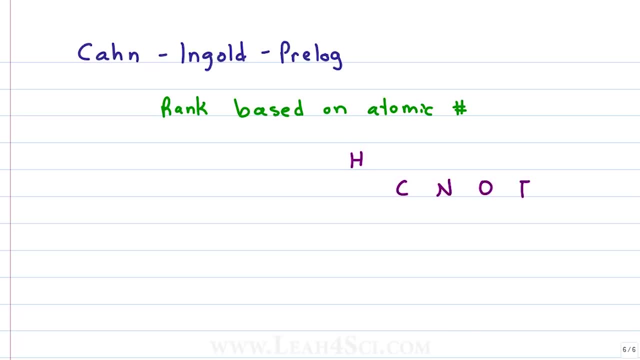 We have hydrogen, then carbon, nitrogen, oxygen, fluorine. below that we have phosphorus, sulfur, chlorine, and then bromine and iodine. These 10 atoms are the most common that you're going to see, especially in a topic like ENZ. As a reminder, iodine is your highest priority. 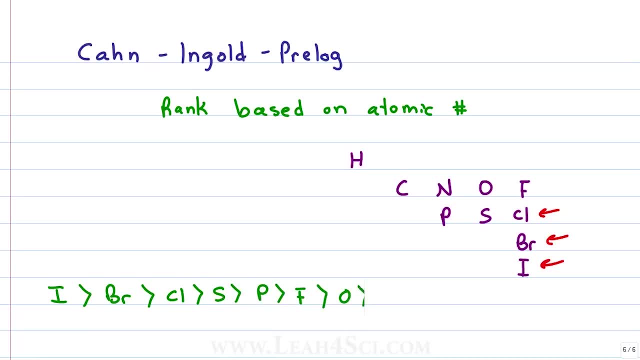 then bromine, then chlorine and sulfur and phosphorus, then fluorine, oxygen, nitrogen, carbon and hydrogen is always your lowest. If there is a difference between these two, let me know in the comments below. deuterium thrown in. remember that it outranks hydrogen because it's just a heavy isotope. 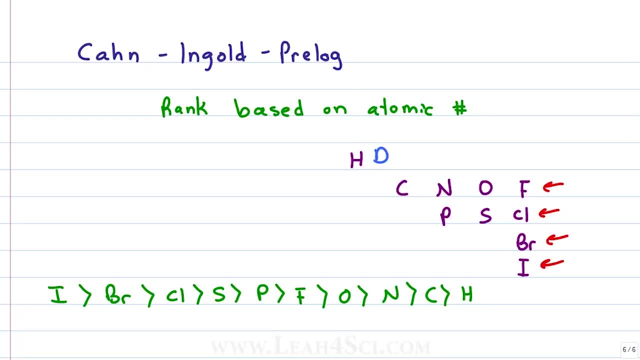 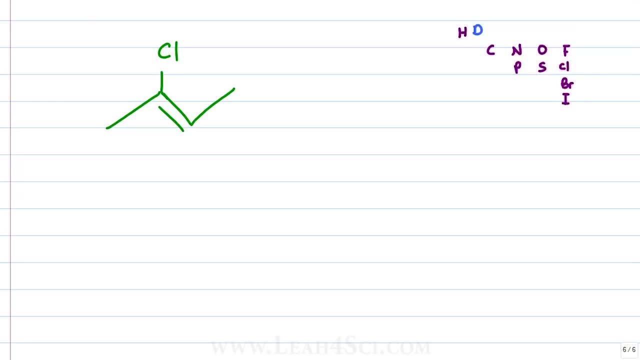 of hydrogen. If you're comfortable with ranking, let's move on. Let's try the chlorine example, and if you haven't memorized the atoms yet, we'll keep it on the side for you. Here's the method that I find to be simplest and least overwhelming. First, identify and highlight. 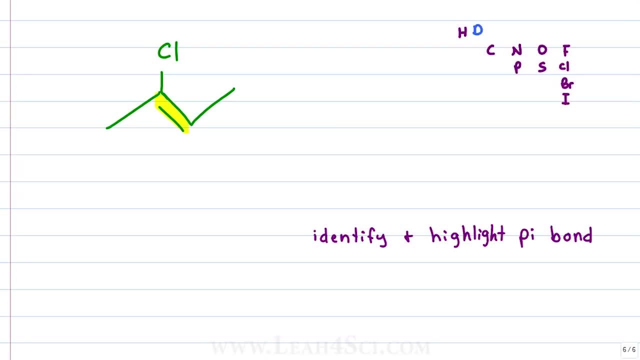 your pi bond, Make it very obvious which two carbons you're looking at and then cover half of the molecule. This is so important because when you have a lot of substituents it's very easy to get overwhelmed and it's very easy to forget what you're looking at. But 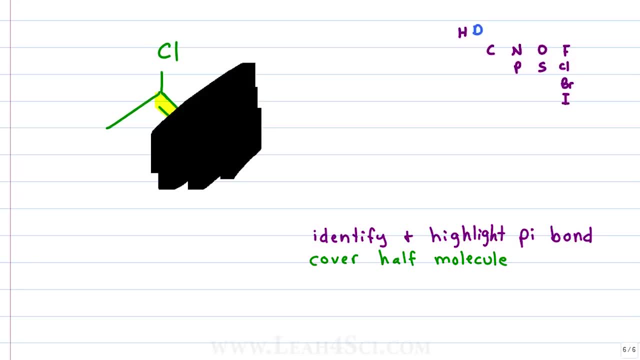 if you cover it by putting your hand or a piece of paper or something, over half of the molecule. you're only focusing on one sp2, one pi bound carbon at a time and keeping it simple. Next, you want to identify the atoms that you're ranking specifically. In this case, we have a chlorine versus a. 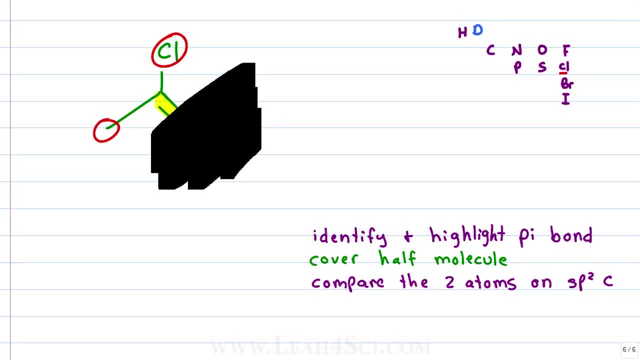 carbon in that methyl group and we see that chlorine outranks carbon. that makes chlorine priority number one and carbon priority number two. Finally, draw an arrow perpendicular to the pi bond in the direction of your higher priority. In this case, my pi bond goes in. 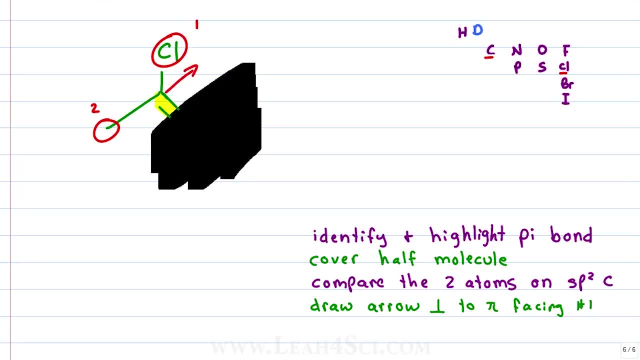 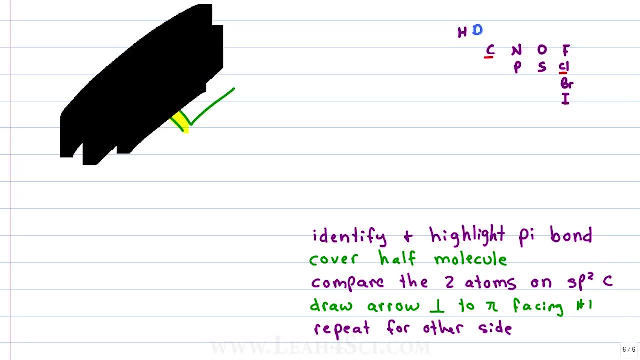 this direction. so I will draw an arrow facing up towards the chlorine. We have one side now we cover it so we're not distracted and do the same thing on the other side. Here's my sp2 carbon, but I only have one substituent. what am I ranking? Don't. 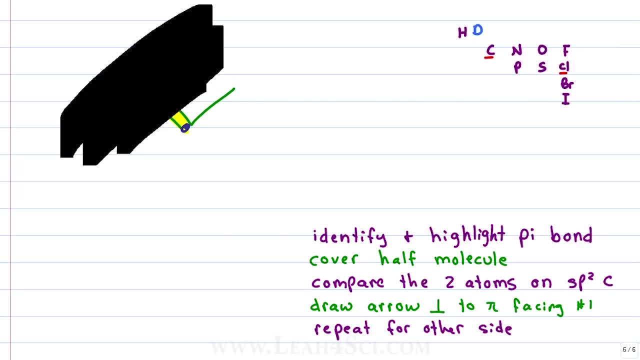 forget that in line structure, hydrogent atoms are invisible, but they're still there. We have a hydrogen atom on this carbon of the pi bond and that means we're ultimately comparing carbon and hydrogen. Carbon will outrank hydrogen, making the methyl group into the pi bond, and 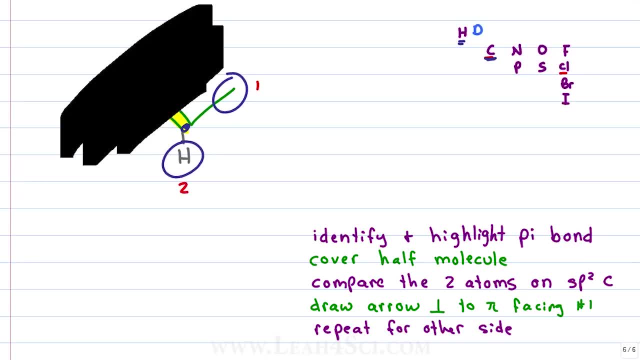 making the methyl group priority number one and the hydrogen priority number two, Since the higher priority is facing up from the pi bond. we'll draw an arrow perpendicular to the pi bond facing priority number one and then uncover both sides. Having the arrows allows you. 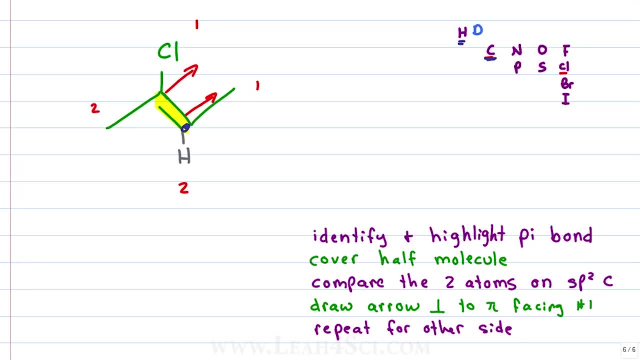 to avoid the groups. It allows you to avoid being overwhelmed and all you have to do is identify: Are your arrows facing in the same direction as we have here, or do you have one arrow facing up and one down in opposite directions? Now be careful, don't call them cis or trans. This is 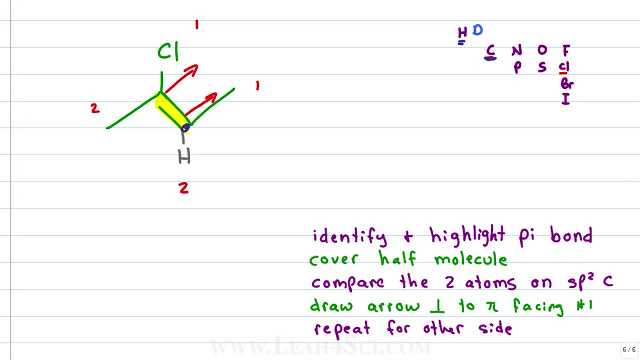 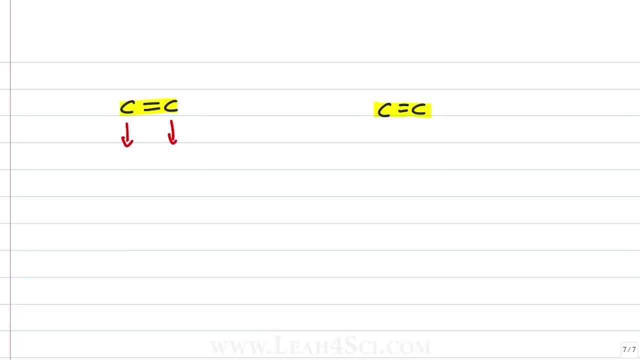 not cis and trans. We're simply looking to see if the two higher priority groups are facing in the same or opposite direction. If you identify that your two arrows are facing in the same direction, this would be the z configuration and the way I remember that. 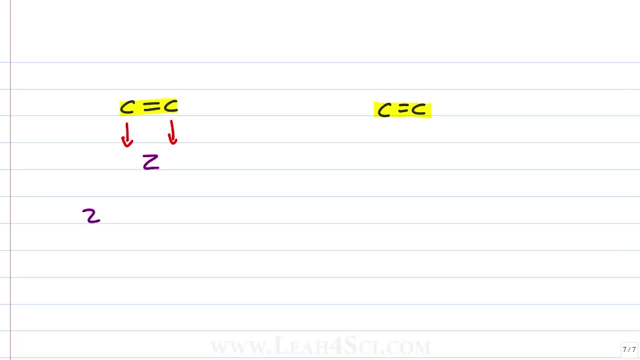 is that I'm going to draw a line that is facing up from the pi bond, facing the same direction. This is by thinking that the two higher priority groups are located on z-zame-zide, all spelled with a z. Z-zame-zide tells me that it's the z configuration If the two high priority groups are. 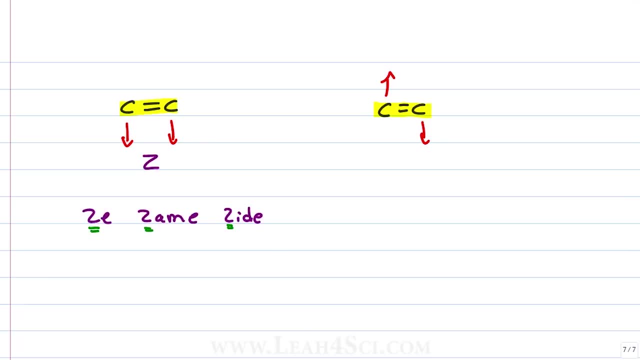 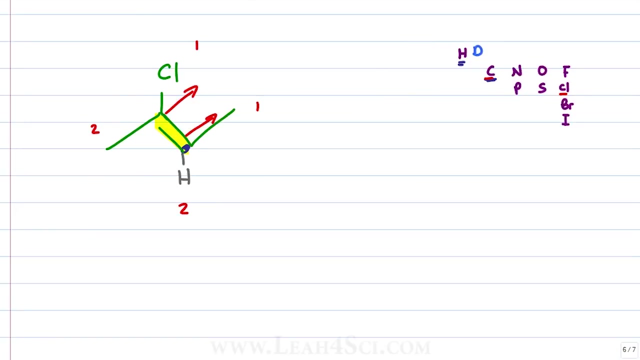 located opposite each other. you get the e configuration and the way I remember it is that these two groups are located opposite from each other, Opposite spelled with an e to remind me they are on e. So these two groups are located opposite sides of each other. Let's go back to our example. In this case. we know that the 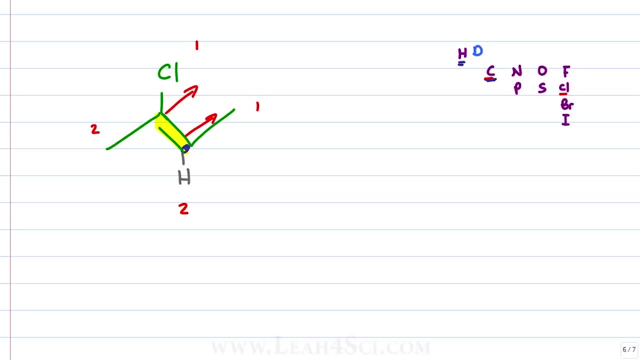 chlorine and methyl, both higher priority, are facing z-zame-zide. That makes this the z configuration To name this molecule. we start with the basic naming rules where we see a total of four carbons in the parent chain for a first name of bute and a pi bond sitting in the middle. 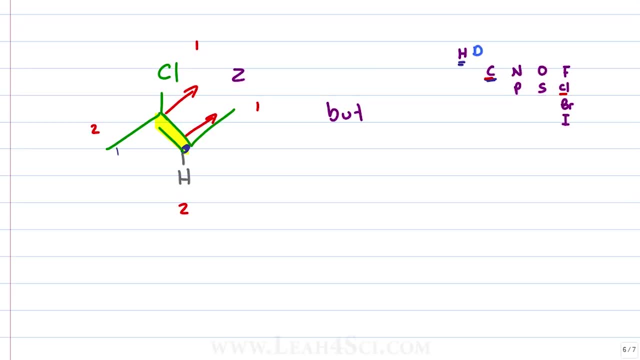 of the molecule. I will number this molecule from the left so that chlorine and the pi bond are both on number two rather than three. Remember, we want the total lowest set of numbers, which gives me a last name of 2-ene and then a chlorine substituent on carbon. 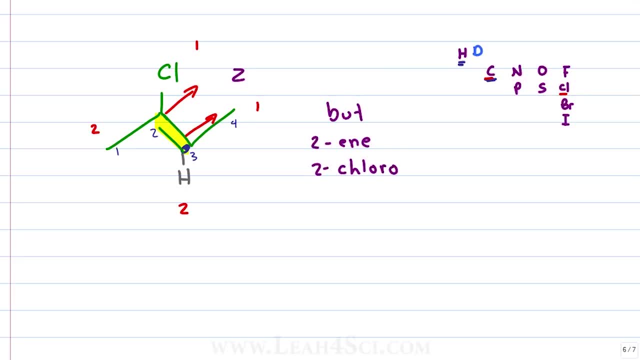 two for 2-chloro. And lastly, we want to include the e-z configuration. In this case, we have z To put the name together. we start with the z at the start of the name and put it into parenthesis, followed by the. 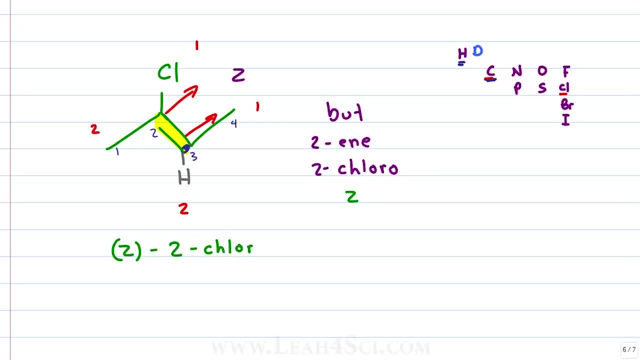 substituent, which is a chloro Chlorine on carbon two. We drag the 2 in front of the bute, giving me two butene. The reason we put the z in parenthesis is to make sure that we don't confuse the letter z with the. 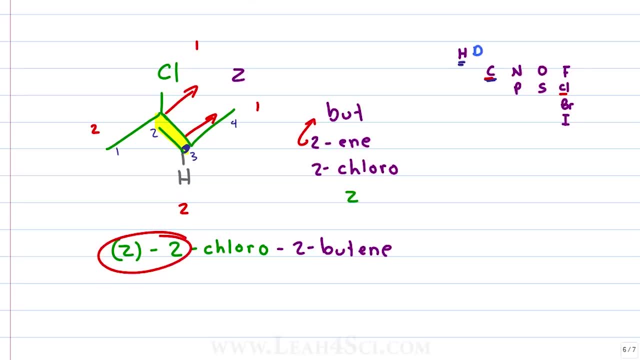 number two. Look at how I've drawn them. they kinda look similar, but having the z in parenthesis reminds us no, this is not a designation of where something shows up. This is z telling me about the stereochemistry or the geometry, about that pi bond. 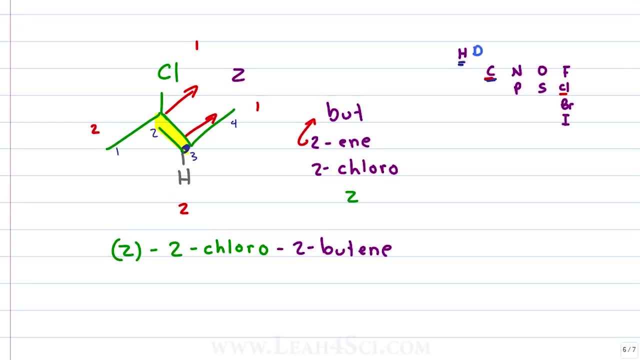 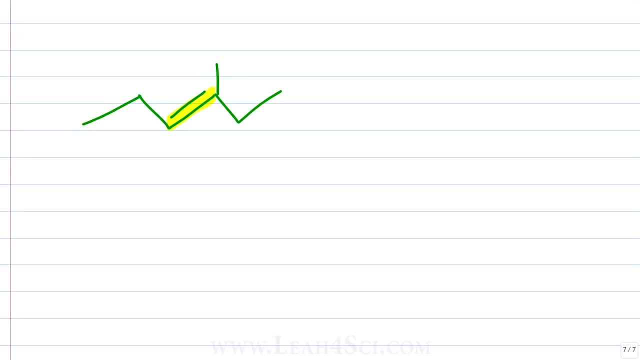 bond for a final name of Z 2-chloro 2-butene. Let's go back and name our first example. We have a total of 6 bonds, giving me a first name of hex. We have an option to number from the right or left. 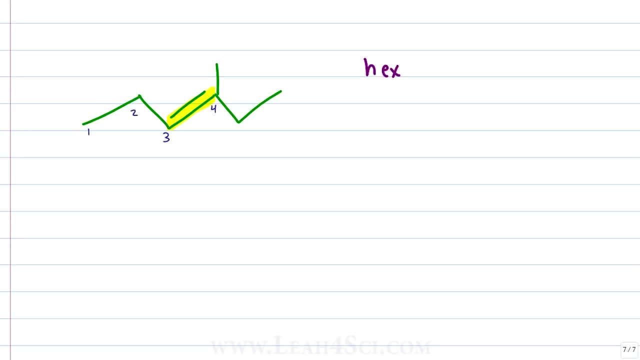 If I numbered from the left, I hit the pi bond at 3 and the methyl group at 4.. If I number from the right, I hit the pi bond and the methyl group at 3 for a total lower set of numbers. So we're gonna choose the red numbering. 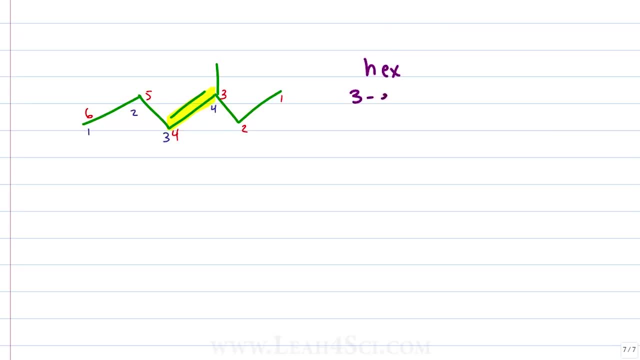 With a pi bond starting at carbon 3, we have 3-ene. A methyl group at carbon 3 gives me 3-methyl. but now we have to specify what's going on with the pi bonds. We don't use cis or trans because we have a methyl and an ethyl. instead we'll use 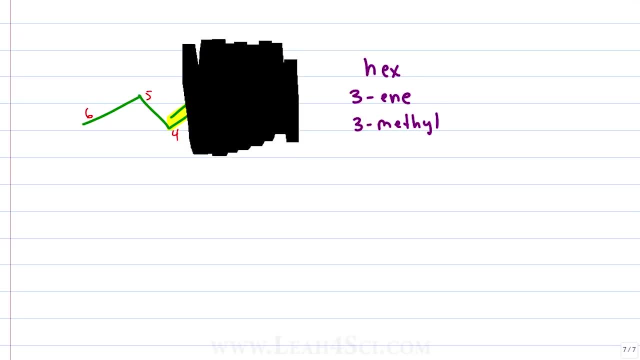 the EZ system. We'll start with the group on the left: identifying the sp2 carbon and recognizing, because the substituent is invisible, there's a hydrogen atom. If you don't have them memorized yet, use this chart as a guide. 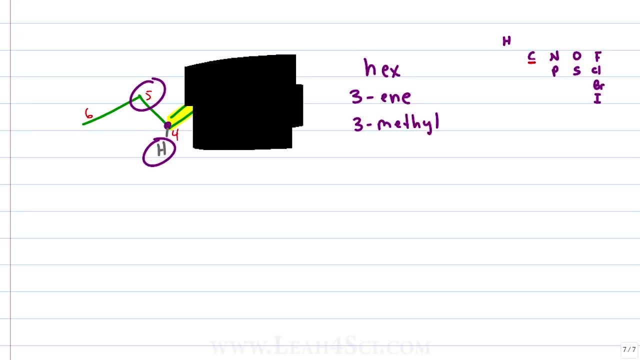 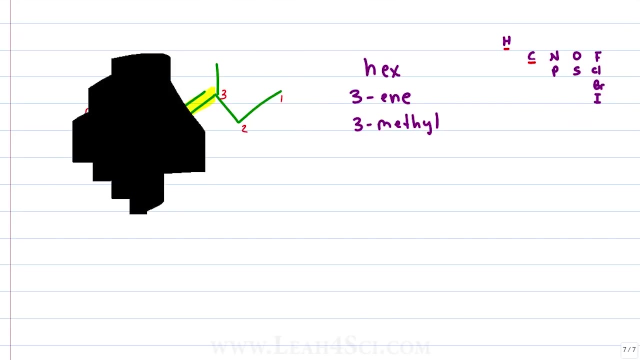 We're comparing carbon to hydrogen. Carbon outranks hydrogen, making the ethyl group priority number 1 and the hydrogen priority number 2, or simply the higher priority in the up direction. Now cover the left side and look at the sp2 carbon on the right. 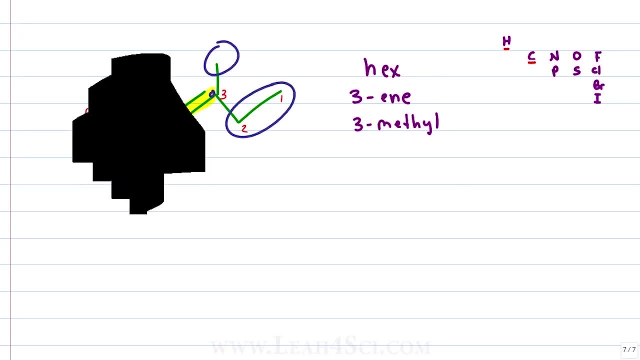 Coming off of this carbon. we have a methyl Methyl and an ethyl Methyl is a CH3, that's carbon. Ethyl is a CH2CH3, that's also carbon. This is where it really helps to understand priority ranking. 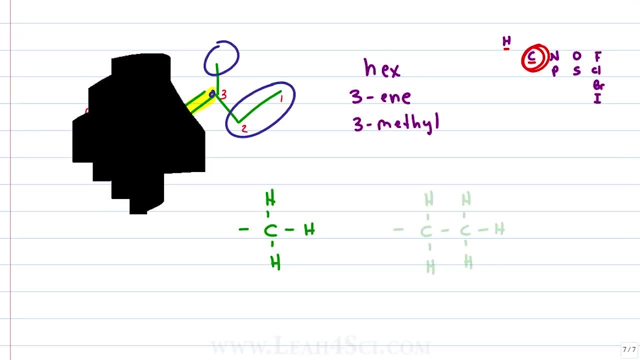 As a reminder, we're dealing with methyl, which is CH3, and ethyl, which is CH2CH3.. We look at the very first atom, which is carbon. since it's the same, we rule it out and go to the next, highest priority. 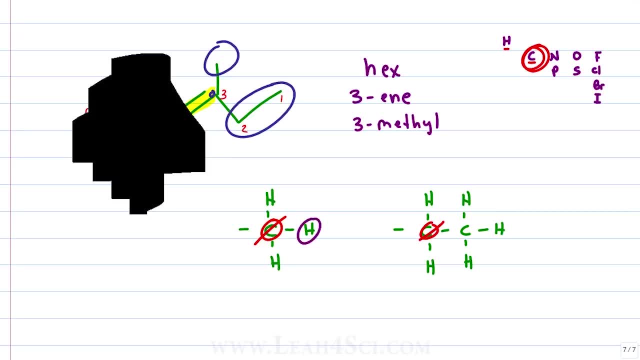 The methyl group has 3-methyl. Let's go to the next highest priority. We have 3 hydrogens, so any one hydrogen is the next high priority. The ethyl group has 2 hydrogens and 1 carbon, but carbon is the highest priority. 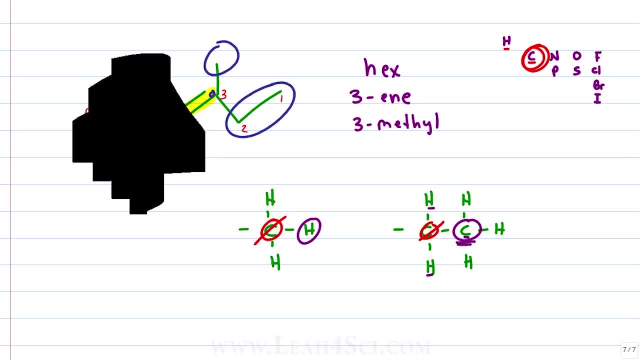 So now we compare carbon to hydrogen carbon wins, making the ethyl group priority group number 1 and the methyl priority number 2.. We'll draw an arrow in the direction of number 1 and then uncover the molecule. Looking at the 2 arrows, they are away from each other. 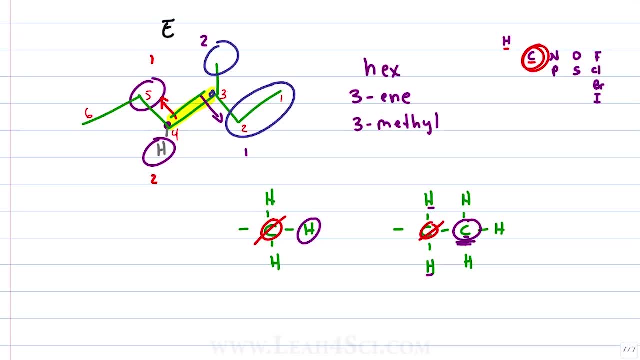 Now I have a molecule which is in the e configuration. Let's put the name together. It's the inhibitor to the emulsifier which is found in the miinus molecule, and we can find it in this molecule. Let's put the name together. 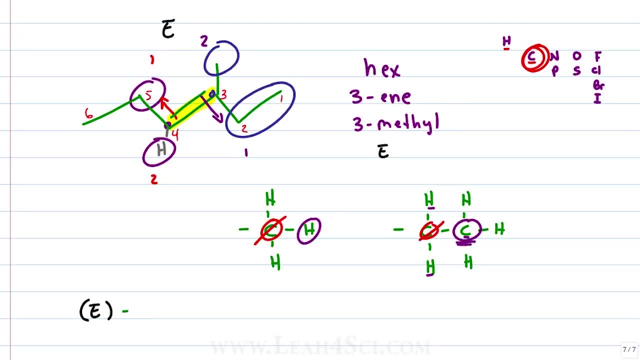 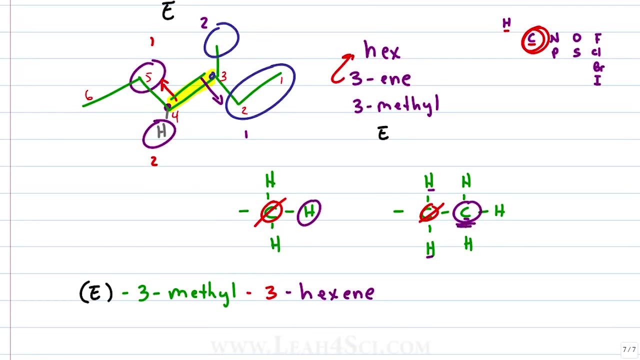 Starting with e in parentheses, followed by the substituent 3-methyl. Pull the 3 in front of hex, giving me 3-hexenes for a final name of E-3-methyl-3-hexenes. Your professor may choose to leave the 3 where it is. in that case, the name would be E-3-methyl-3-hexenes. 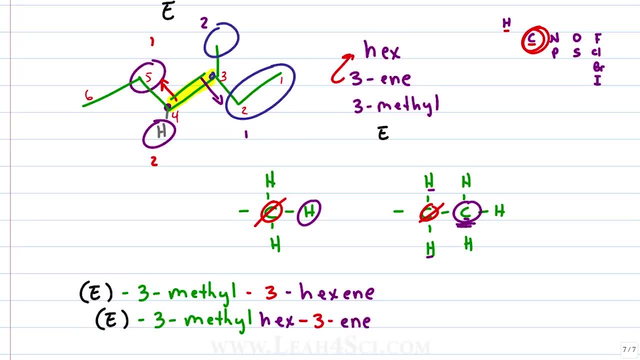 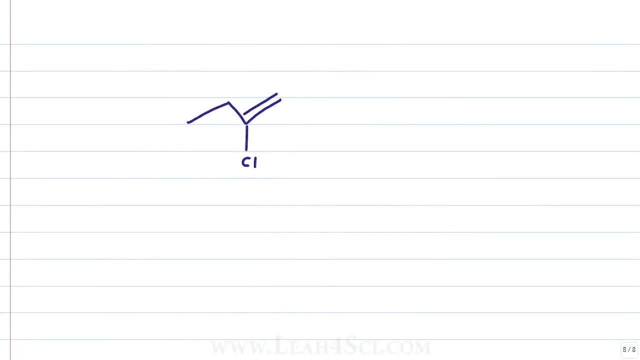 Both are accurate. Thank you are correct. What about a molecule that looks like this? We have a pi bond with two unique substituents. If we look at the sp2 carbon, on the left, chlorine outranks ethyl, making the chlorine higher priority, but on the right, we don't appear to have anything, meaning we 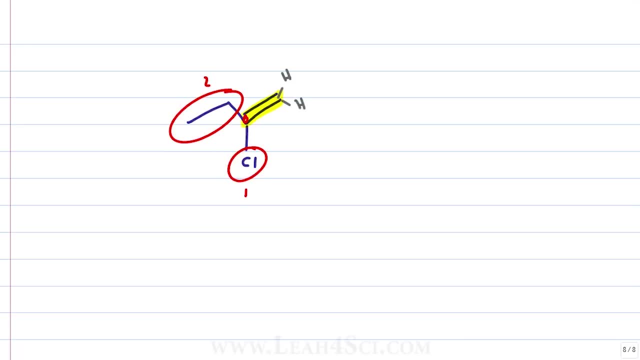 have two hidden hydrogen atoms, but once again, like we saw in the last video, hydrogen is the same as hydrogen. If you have two equal priority groups, one doesn't outrank the other, and that means there is no stereoisomerism here, because there's no way to differentiate.